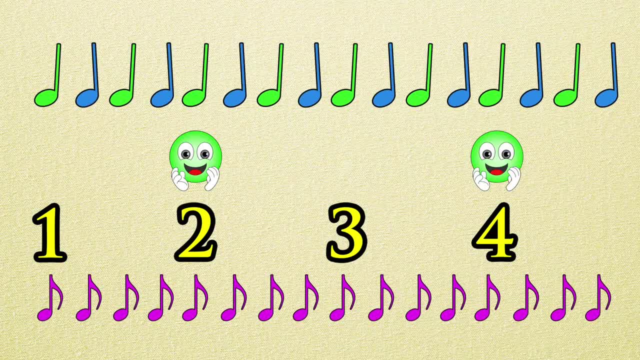 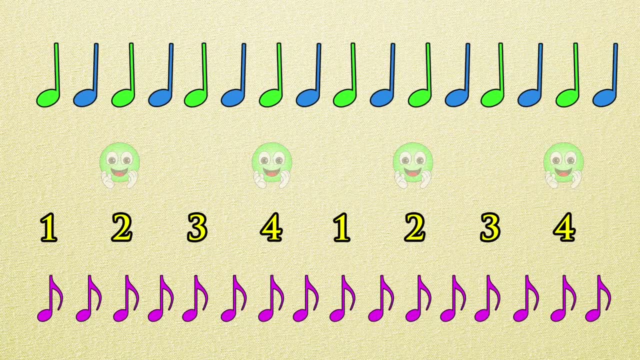 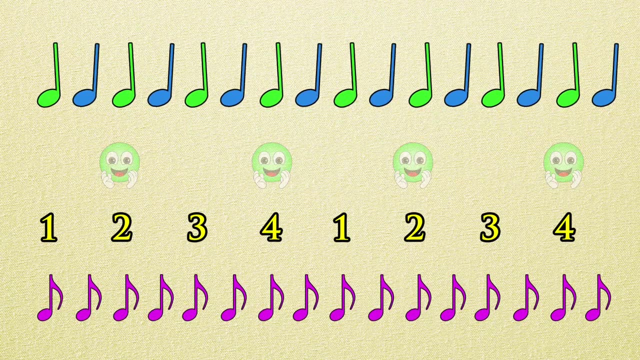 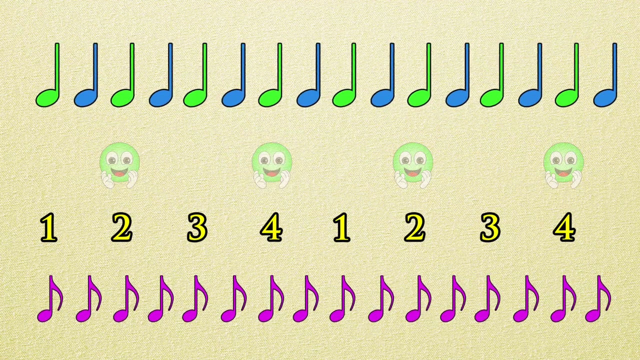 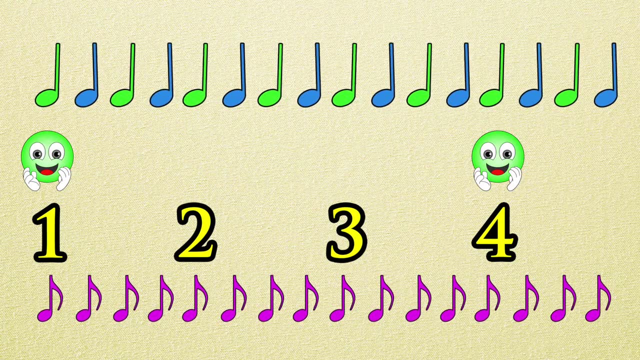 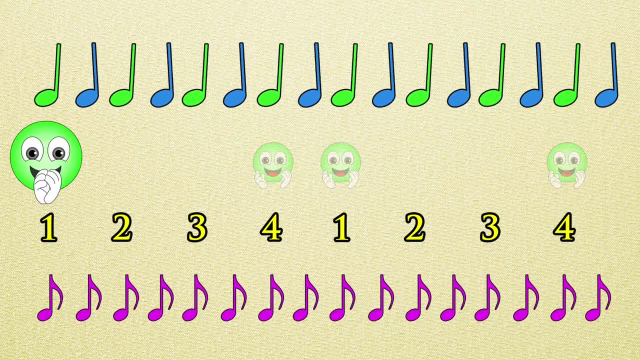 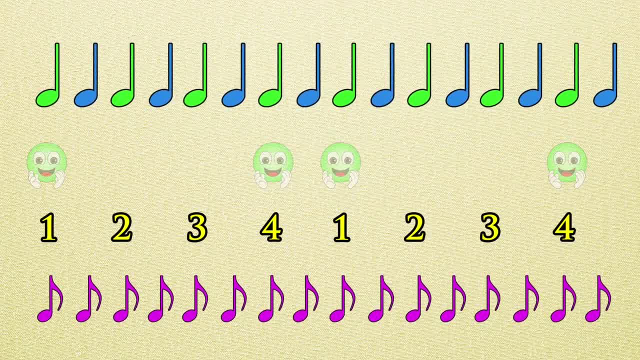 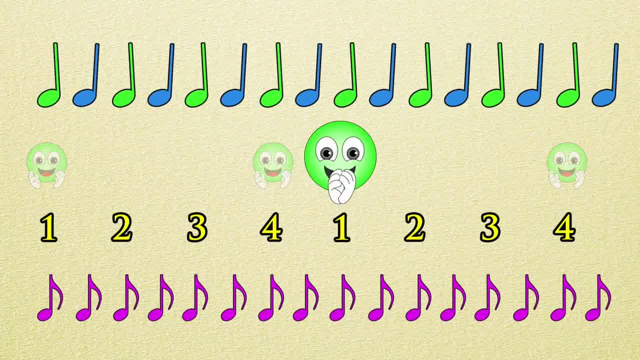 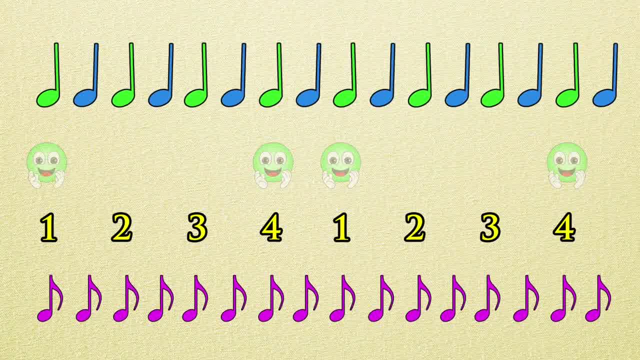 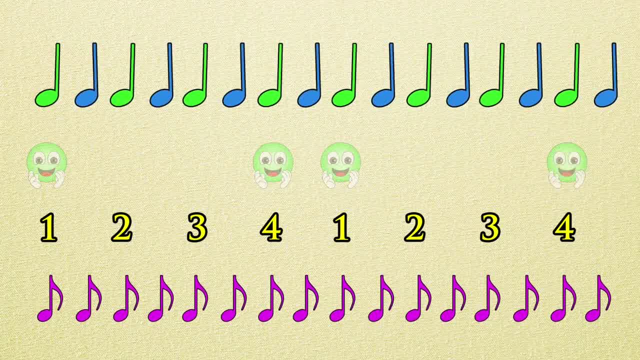 we've got rock and we clap in beats 2 and 4.. Great, Now let's switch to eastern music. This time we will clap in beats 1 and 4.. Ah, why don't we relax a bit more now and play some reggae from the Caribbean Again? 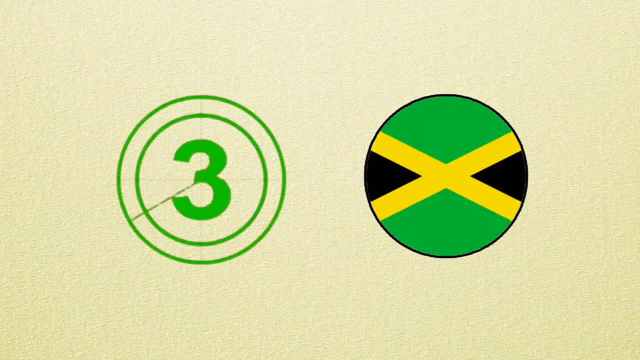 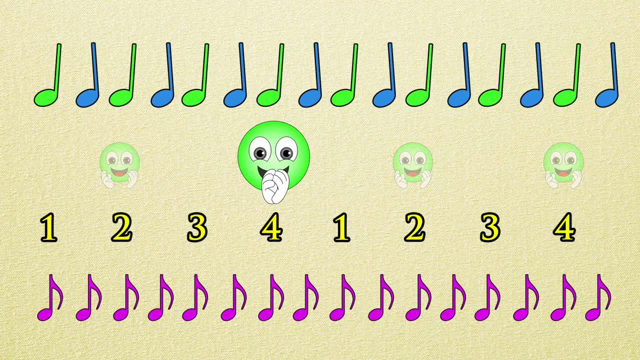 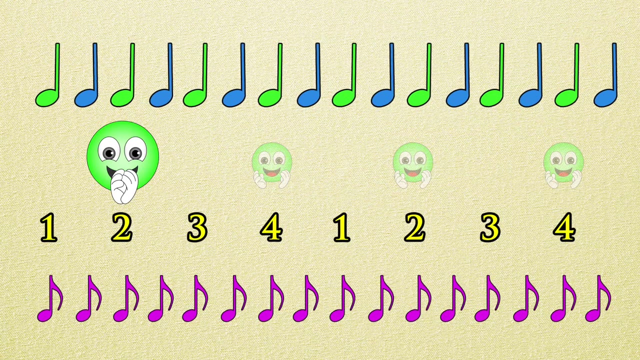 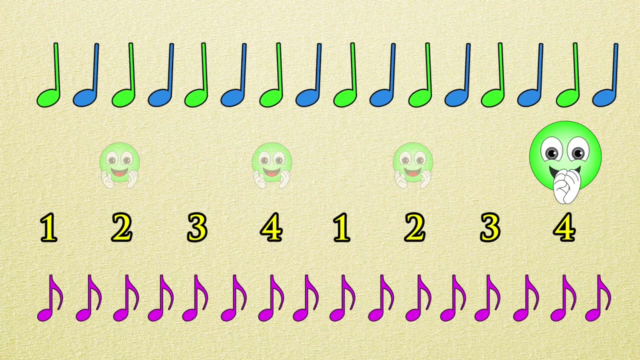 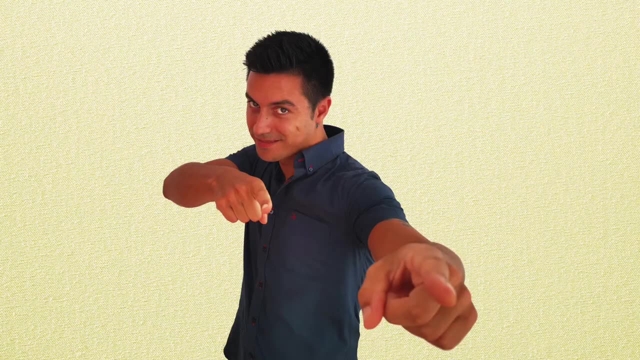 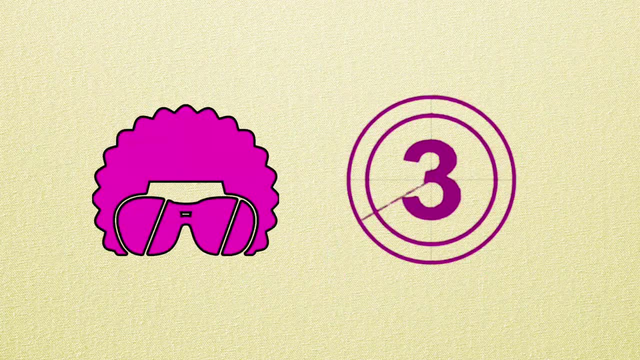 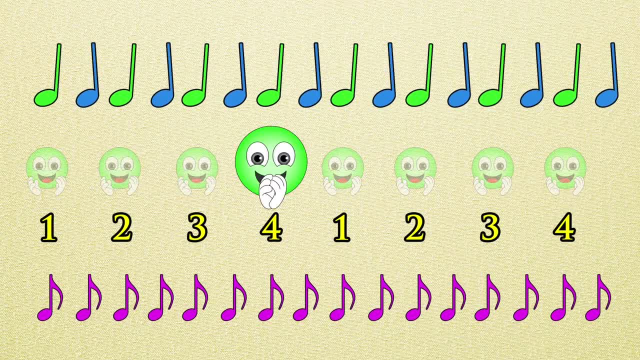 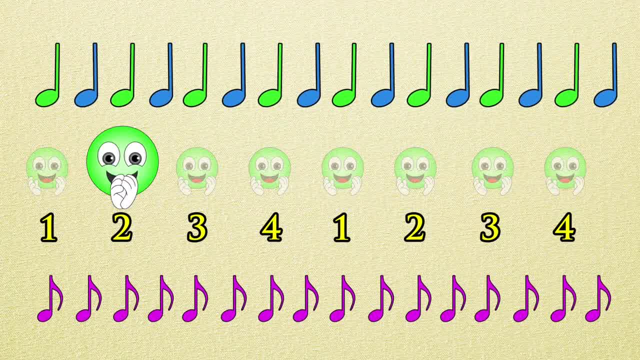 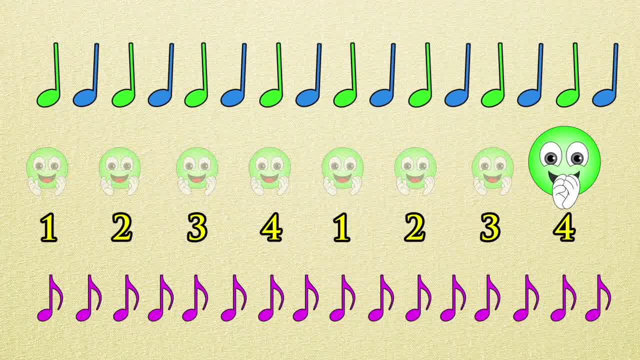 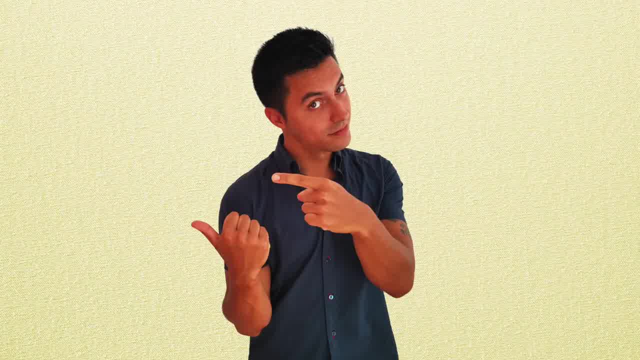 we clap on beats 2 and 4.. Now we will play some reggae from the Caribbean. all right, all right, let's funk this up, get up and dance, clap on beats one, two, three and four and we go back to relaxing with some smooth jazz. this time we will clap the hi-hat. just follow me. 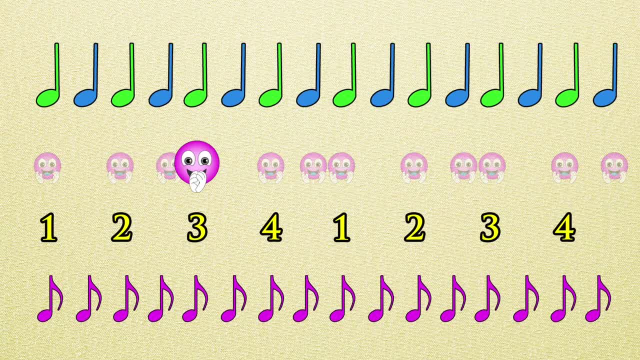 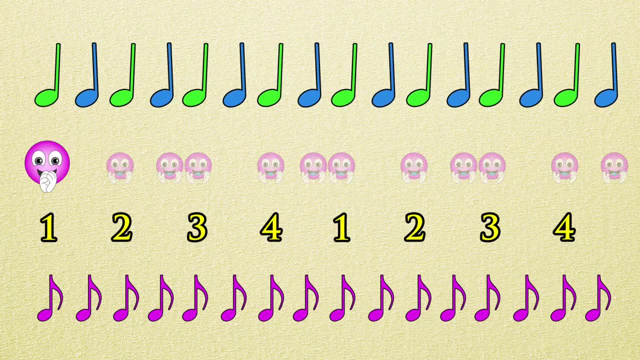 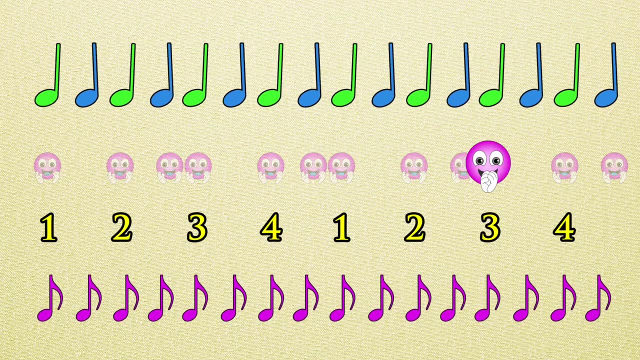 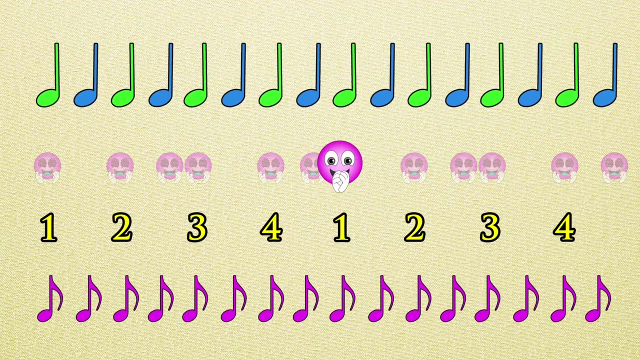 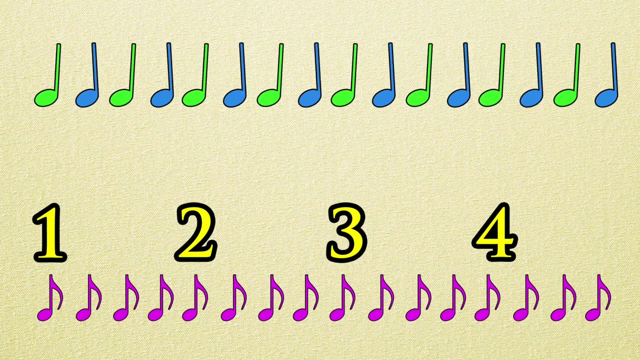 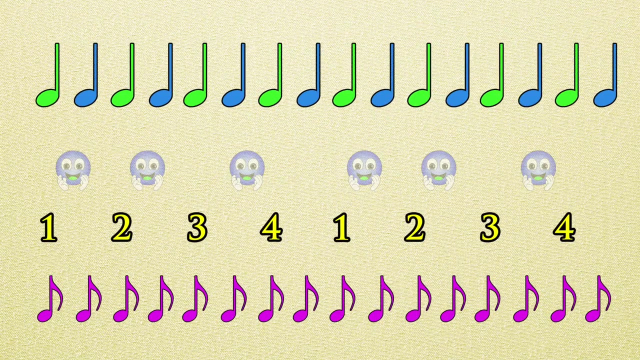 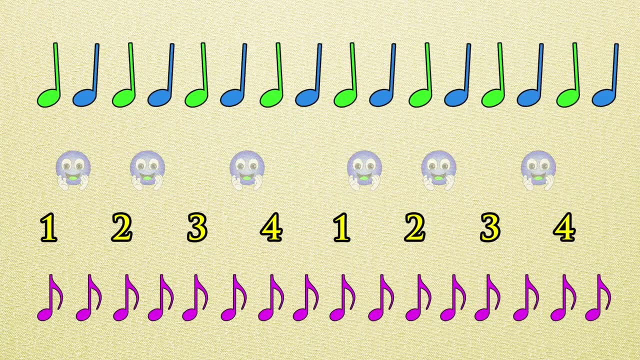 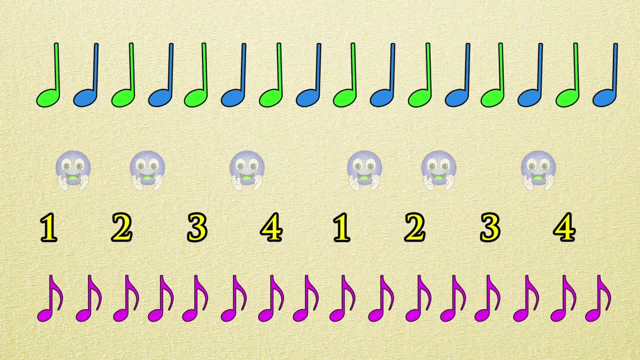 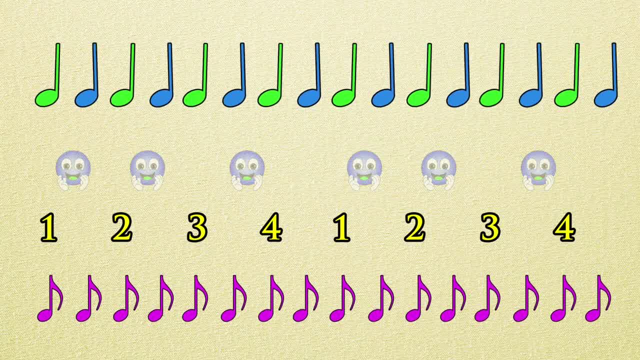 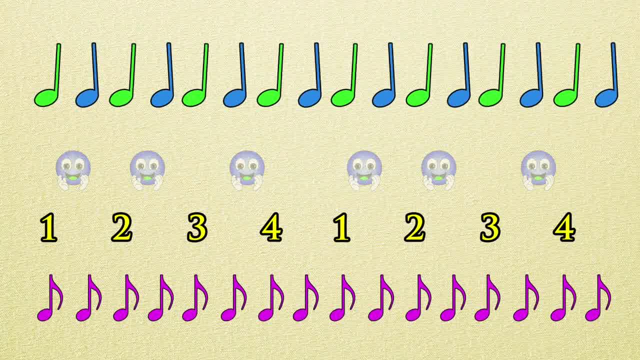 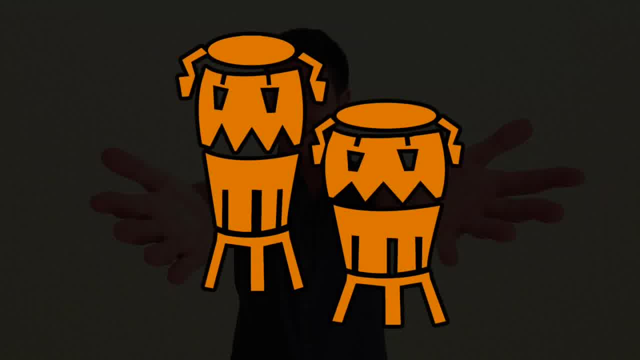 now we'll play some electronic music. this is the hi-hat. it's beginning to get tricky. we will clap after the first and second beats, then just before the fourth, did you get it? the next one is a modern latin beat. i'm sure you recognize it. 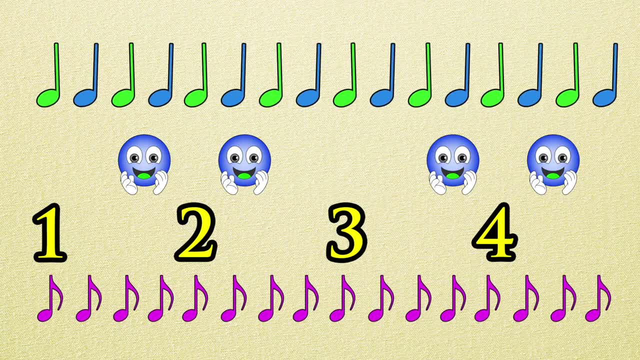 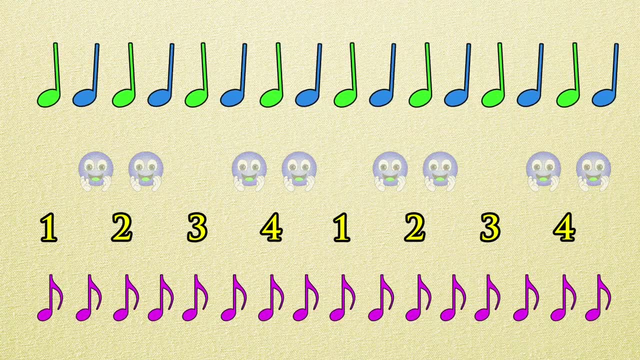 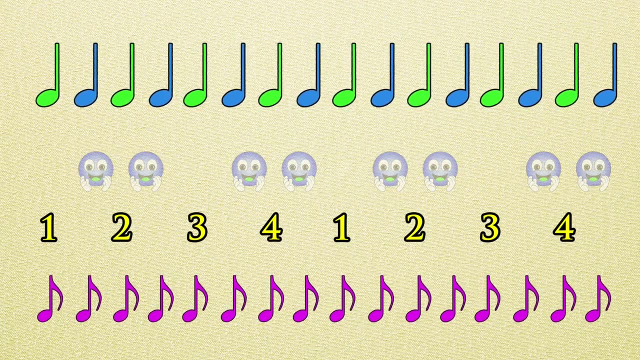 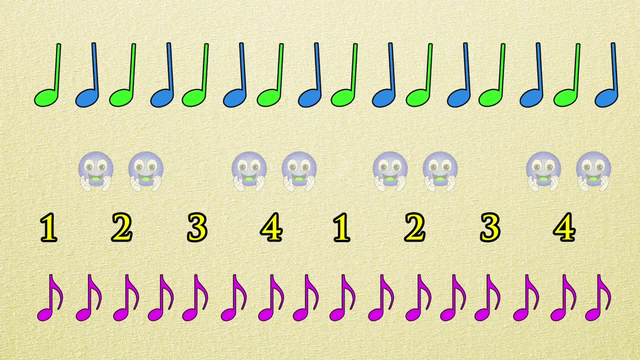 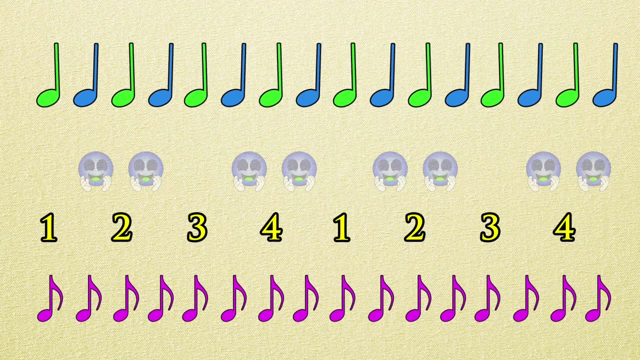 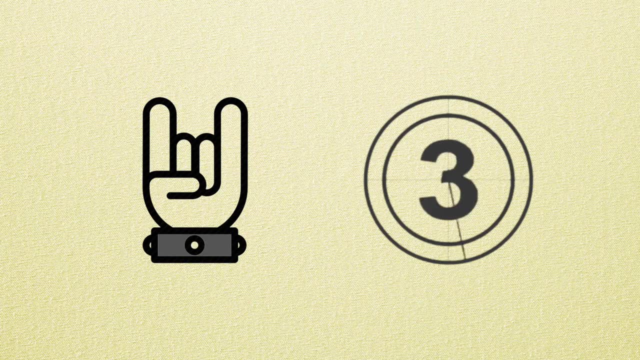 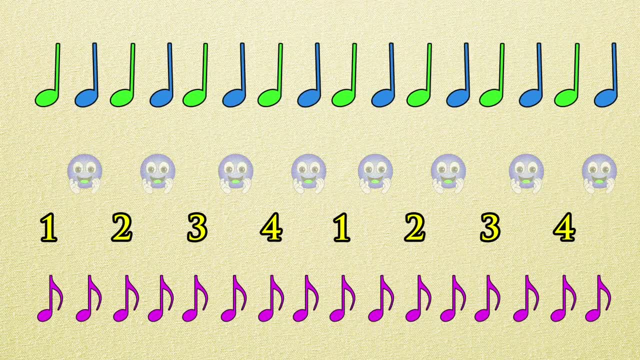 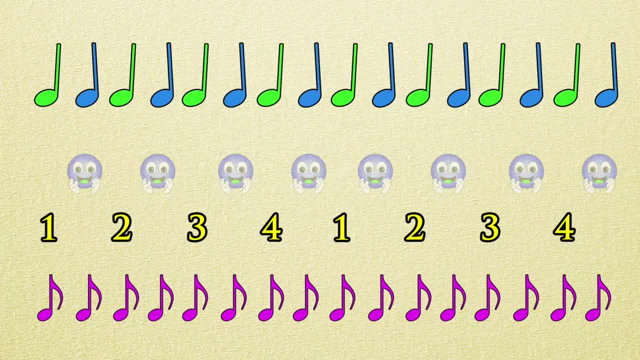 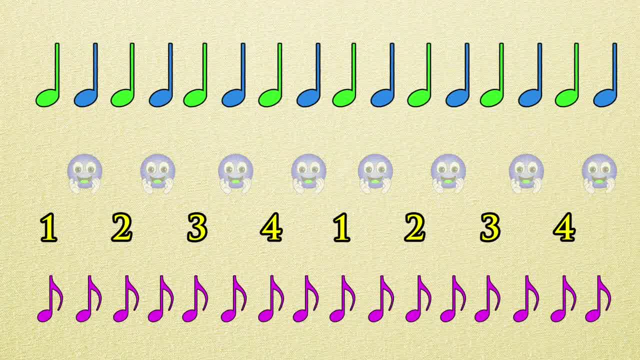 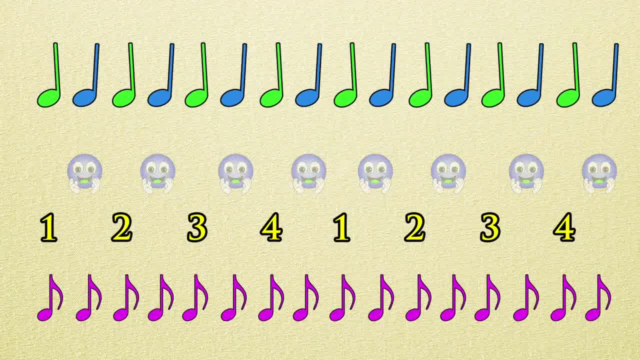 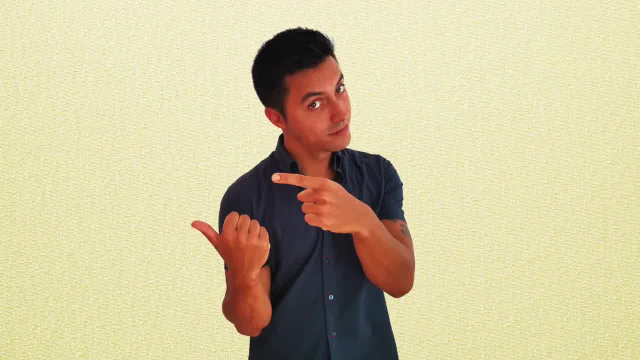 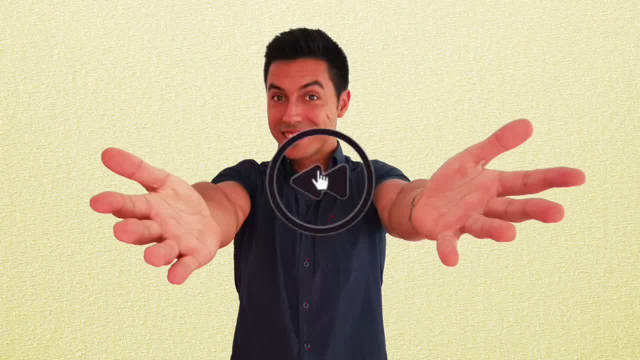 focus on beats two and four. there's a clap before and after each one of them, and we will finish with some offbeat metal music. you have to clap always on the offbeat. so Wow, that was something else, wasn't it? Our ClapClap game is over now, but you can always play again as many times as you want. 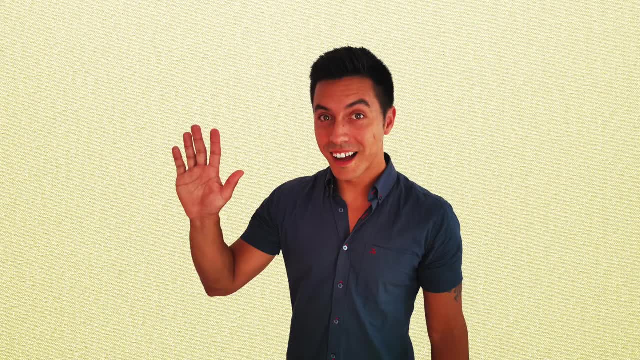 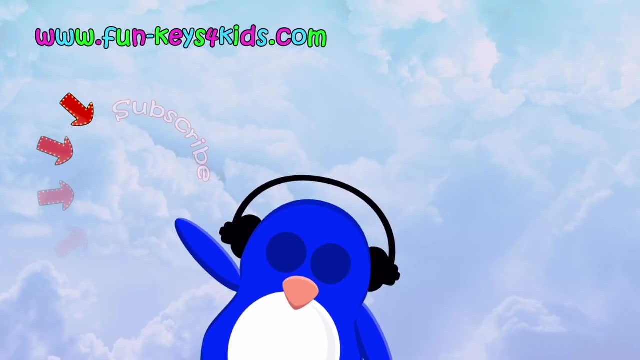 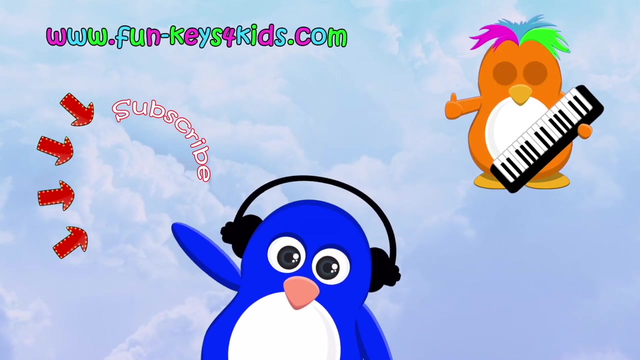 Just go back to the beginning of the video. See you soon with more ClapClap games. Don't forget to subscribe. See you soon with more ClapClap games.